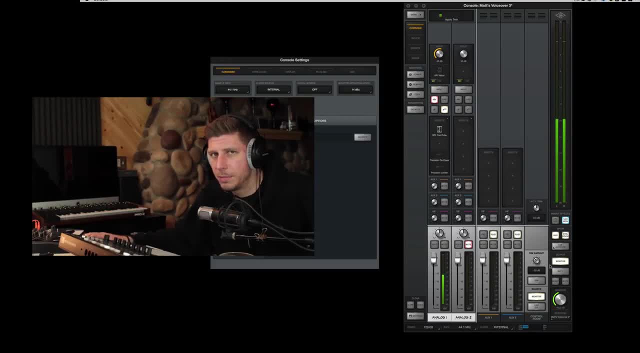 and basically reference my mix on a second pair of speakers or monitors. So that's it. Hope it was helpful Straight into the point. Take care, Oh and thank you. Universal Audio- This console too is amazing. 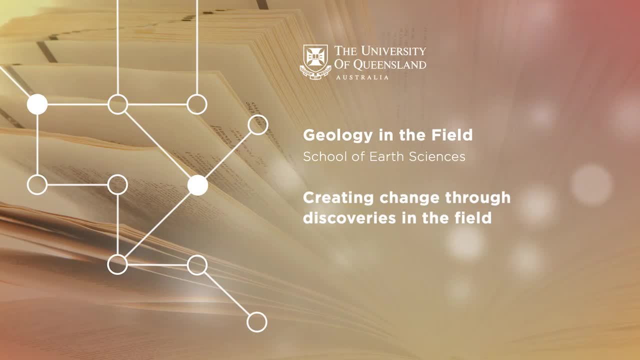 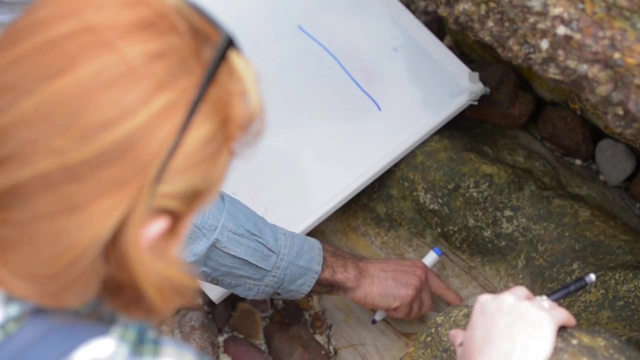 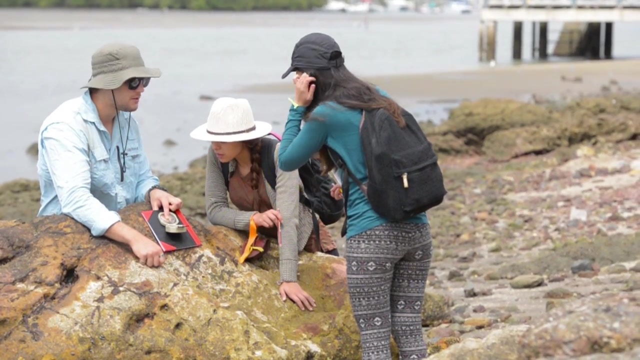 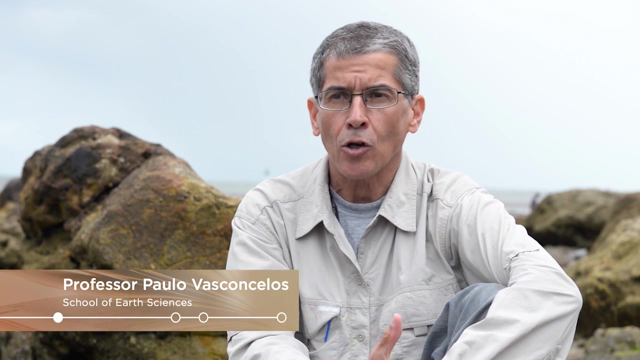 From rocks to reefs. geology is not just about observation, but also measurement, interpretation and synthesis. The School of Earth Sciences has developed an innovative teaching program with a focus on hands-on discovery in the field. Through the years, we realized that most of the students really learn much more when they are 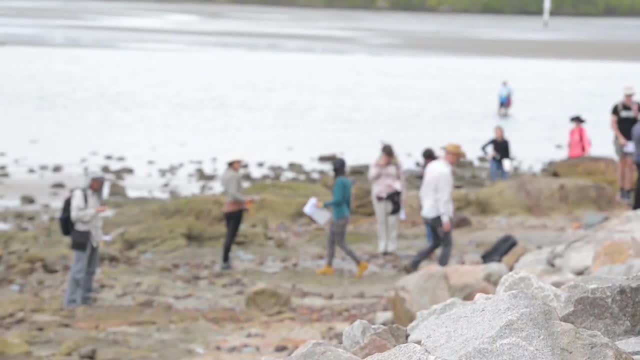 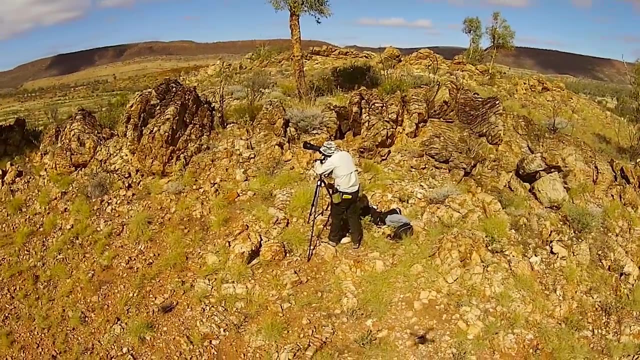 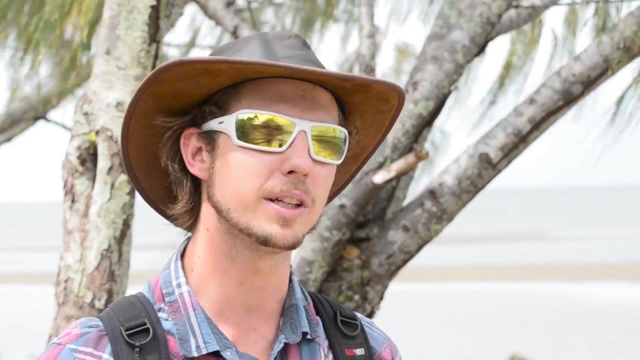 in a field situation than they do in a classroom. It's one thing to see theoretical experimental data and to look at the papers about all the different things we study, but when you go to the field and you actually see it, those little pieces of information unlock the story. That's what's really cool about field geology. 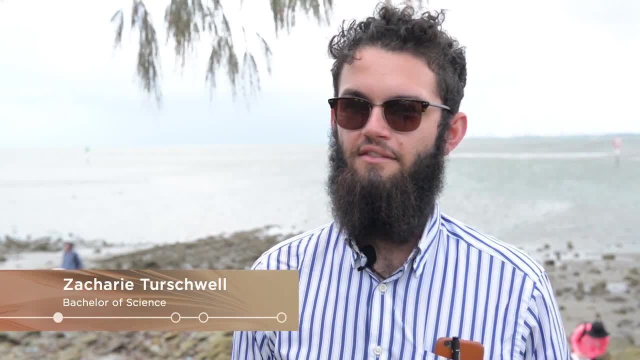 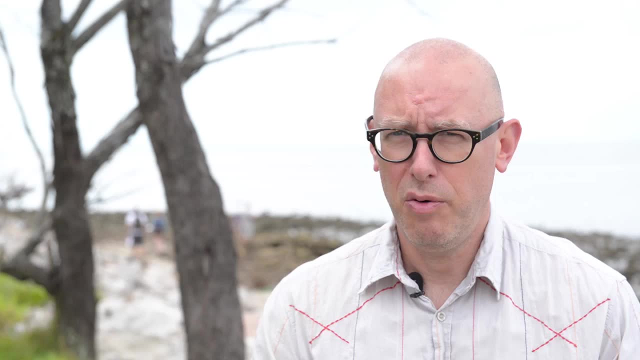 You're actually seeing the rocks, getting this hands-on experience with taking the physical measurements And really getting a good image of what's happened here geologically. So what we're trying to do is finding better ways to expose the students to the field experience. 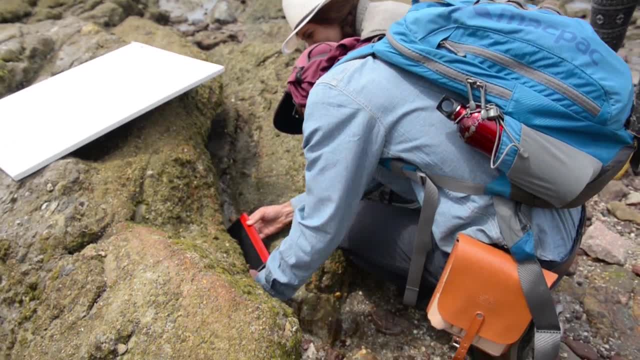 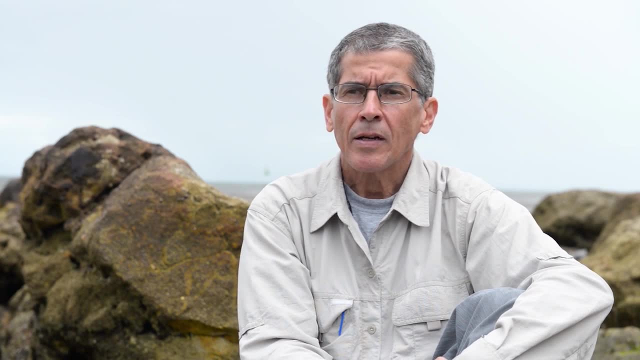 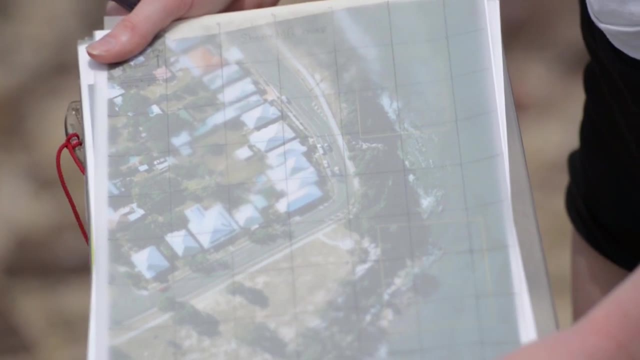 which is what they really need to develop their skills. Our students are actually very well trained When they go into industry. they actually are recognized for their competence in the field. Industry recognizes the value that we have in their education And that's what we're trying to do. 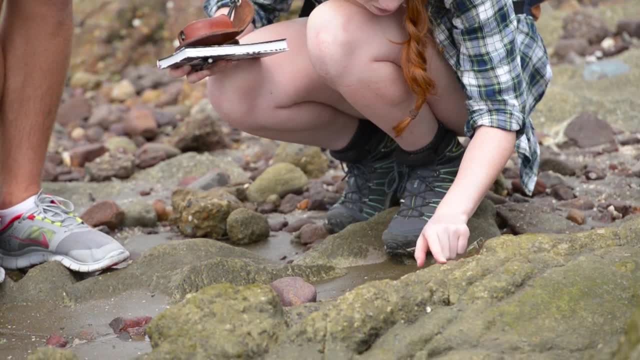 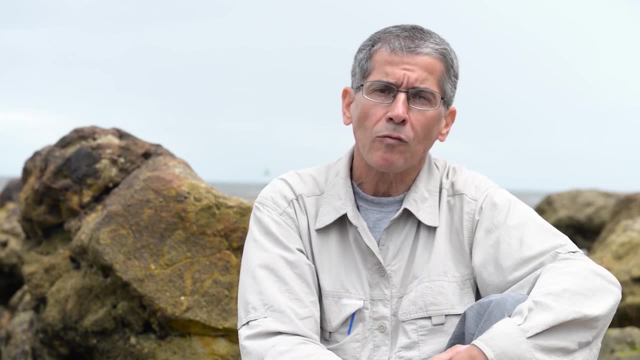 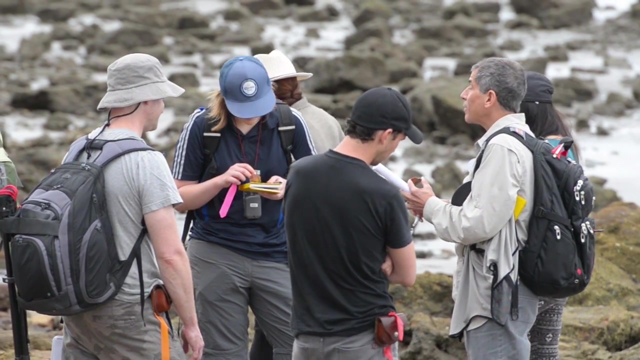 They're actually developing partnerships with us. In the last couple of years, Rio Tinto has employed a number of our students. It's a win-win situation both for industry and for the academic institution. So we work very hard to do things in an innovative way, in an engaging way, in a program that 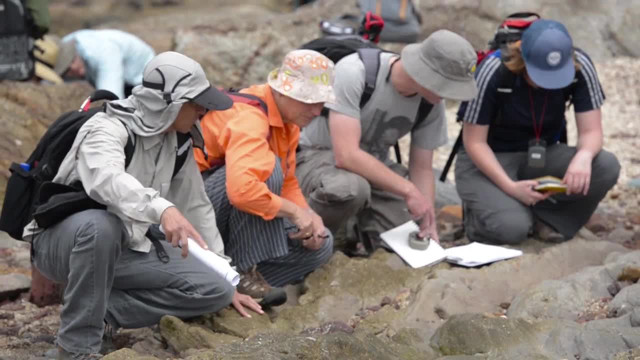 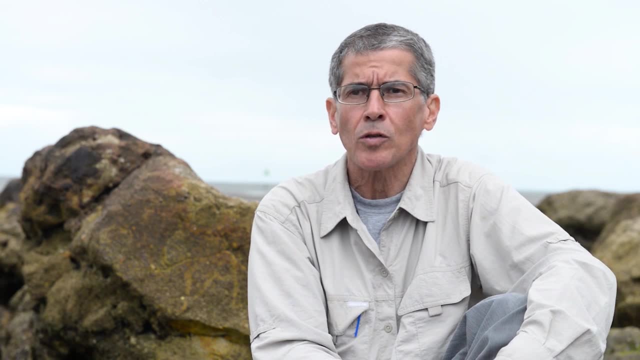 actually gives our students a career path that actually will be very successful into the future, And that's what we're trying to do, And that's what we're trying to do And that's something we're very proud of. UQ has produced a very large number of very successful geologists in Australia, and I